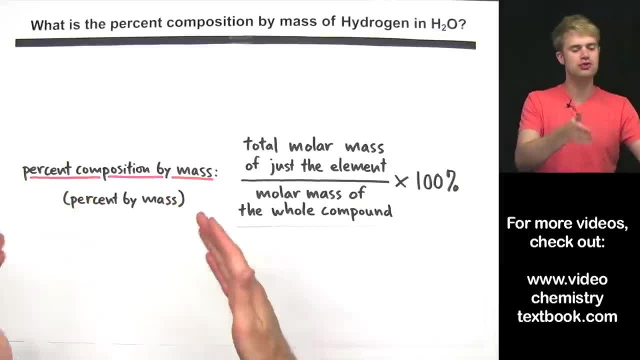 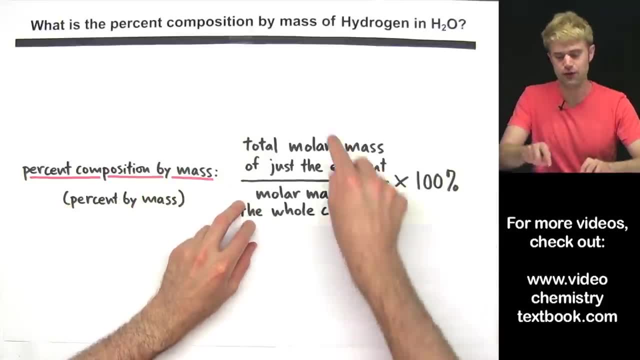 And just so you know, sometimes percent composition by mass is referred to only as percent by mass. They're the same thing. Okay, so here's our equation, and it's got a big fraction. The fraction's got a top and a bottom. So on the top of the fraction we have the total molar mass of 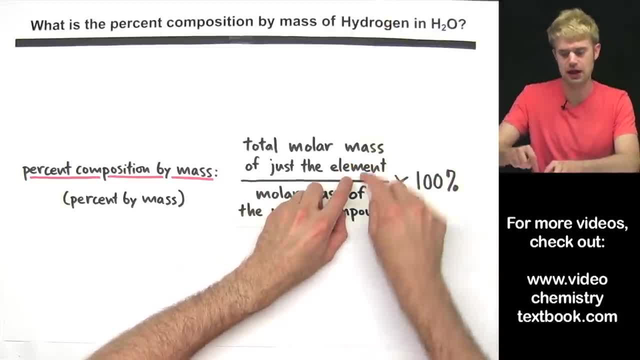 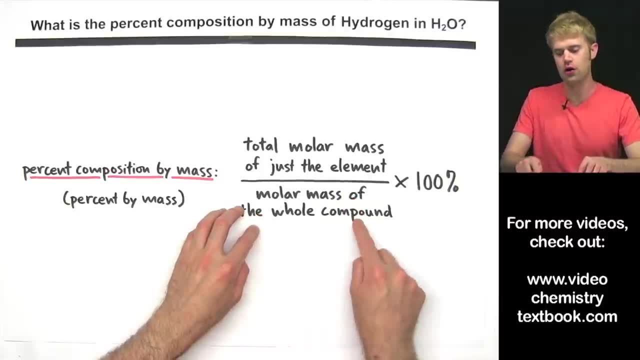 just the element. In this case, hydrogen is the element, and I'm going to talk more about the top of the fraction in a minute. on the bottom of the fraction, we have the molar mass of the whole compound. in this case, the compound is water. We're going to do some division. we're going to 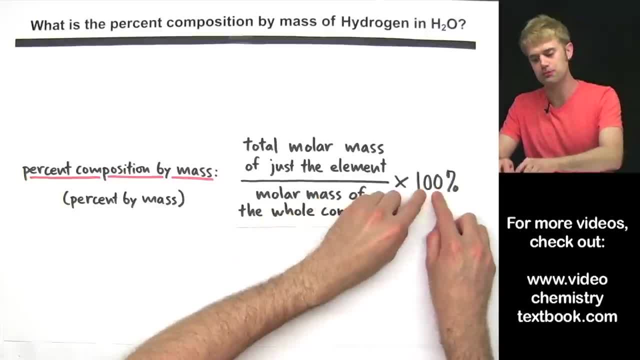 divide the top by the bottom, and then we're going to take that and multiply it by 100%. Okay so, to start solving for this, we're going to start taking the fraction by its bonunder population. Okay so, to start solving for this, we're. 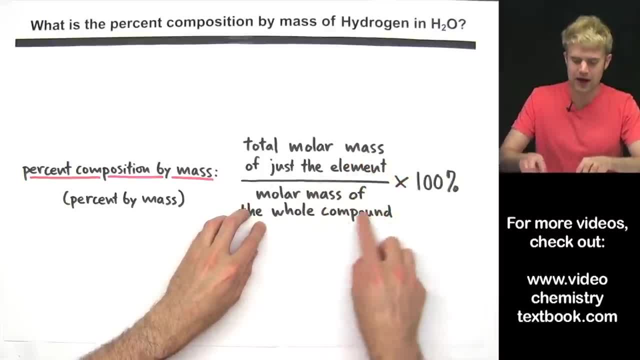 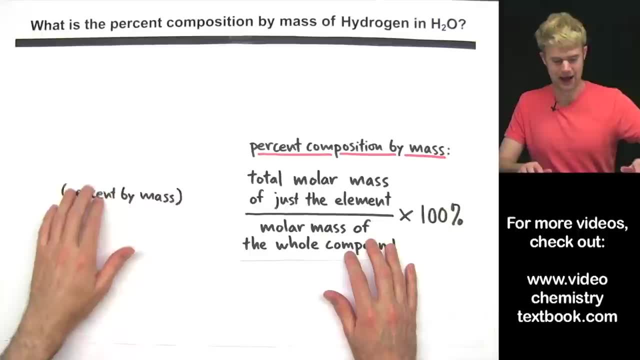 We are going to want to get a number for the top and we're going to want to get a number for the bottom. here Let's start on the bottom. okay, Let's start by calculating the molar mass of H2O of water. 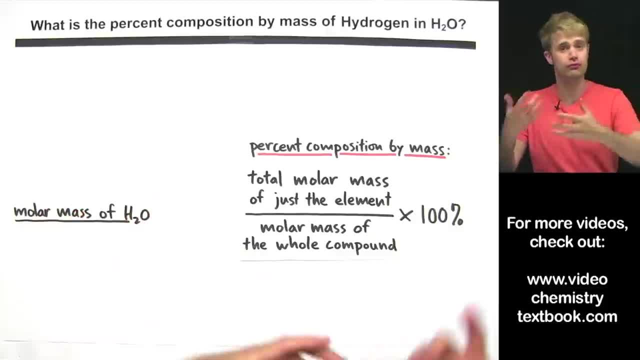 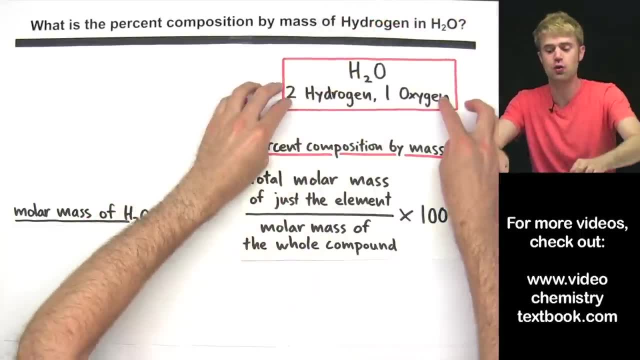 Now you may already know how to calculate molar mass. If you need a refresher, I got a video on that. But just real quick, what we're going to do is we're going to look at the chemical formula here for H2O. 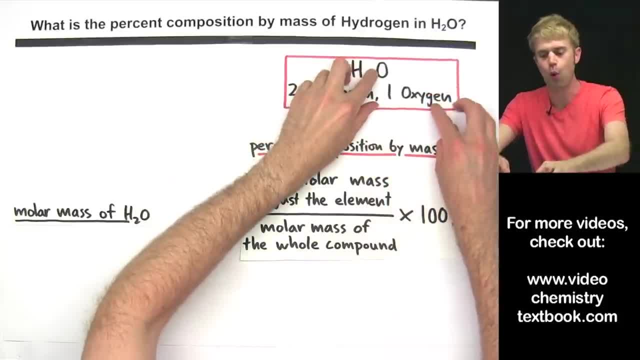 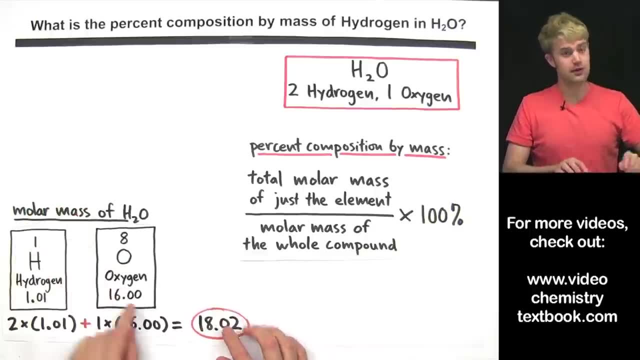 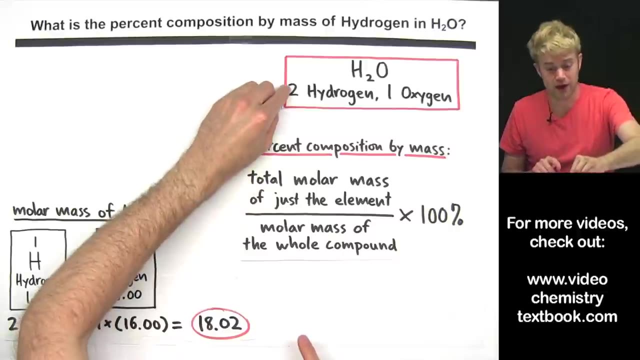 which tells us that there are two hydrogens and one oxygen. okay, Okay, so then we will look up hydrogen and oxygen on the periodic table. okay, This number here- 1.01, tells us the molar mass of hydrogen, and we got two of them. 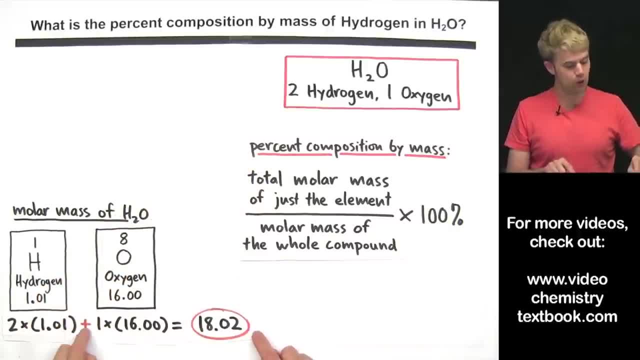 So we do two times this number and then we add it to one, because we have one oxygen, one times the molar mass of oxygen. We do the addition and we get 18.02, the molar mass of H2O, which is how much one. 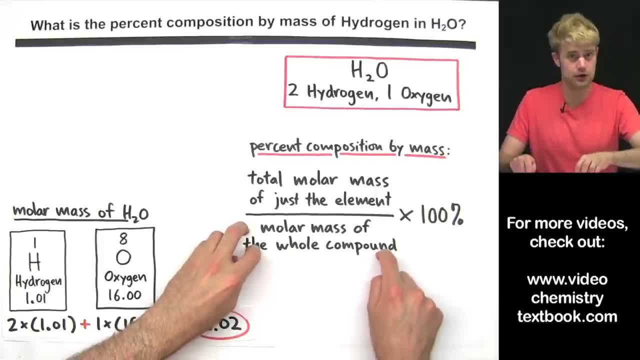 One mole of H2O would weigh, okay. So that's the bottom here of the fraction. Now let's talk about the top here. okay, What do I mean when I say the total molar mass of just the element? Okay, well, when we calculated the molar mass of H2O, 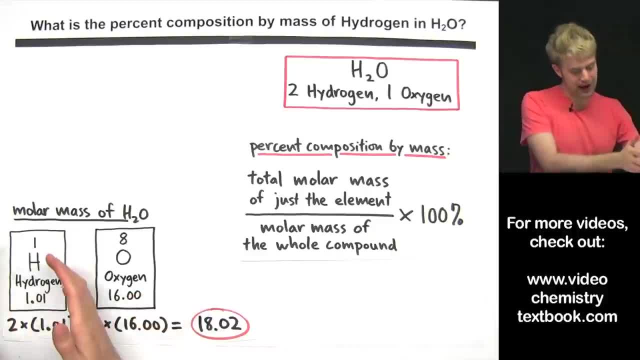 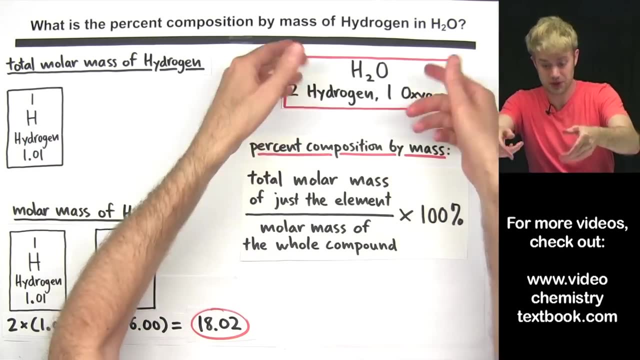 we added together the molar masses of hydrogen and of oxygen. We combined both of these, But I want to find out the total molar mass of just the hydrogen, not both of these things added together. All right, So if we look at the equation here, I mean sorry, 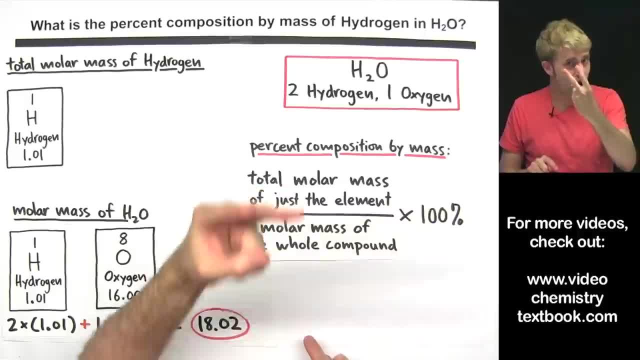 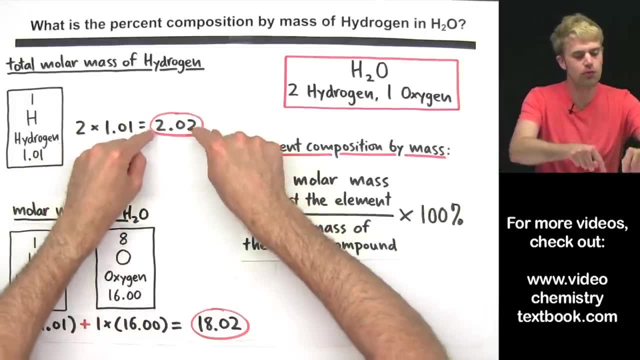 if we look at the formula here, we see that we have two hydrogens. okay, Each one weighs this much, So we do two times 1.01 to get the total molar mass of just the hydrogen. okay, This is the total molar mass of the hydrogen on its own. 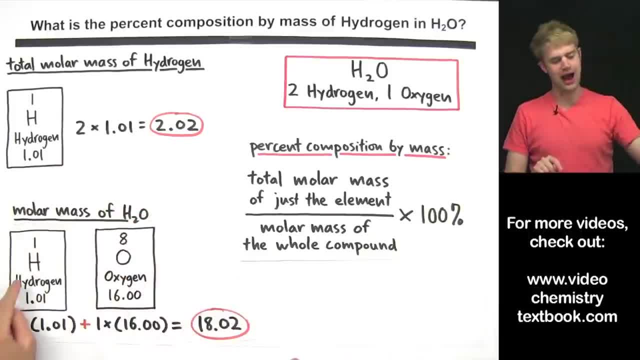 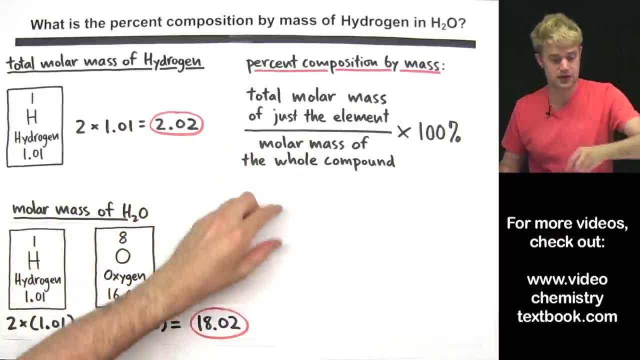 and this is the total molar mass of everything the hydrogen added to the oxygen. So now we can take these values and plug them into the equation. okay, So on the top, the total molar mass of just the hydrogen is going to be 2.02.. 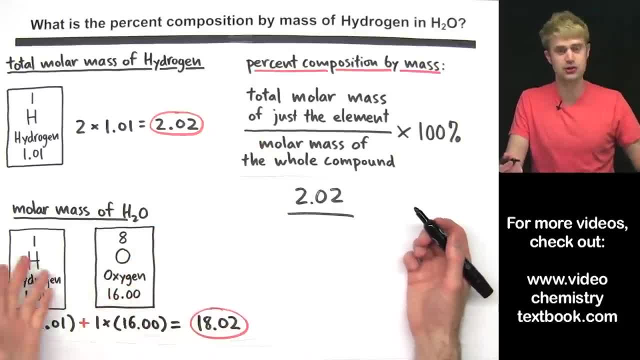 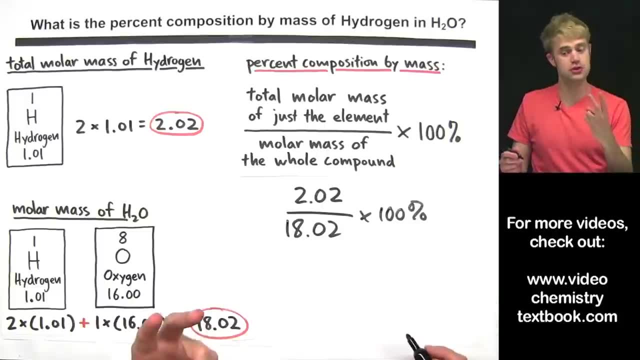 And then on the bottom, the molar mass of the whole compound of the hydrogen and oxygen added together of the water is going to be 18.02 times 100%. I'll do this in two steps, okay. So the first step, just doing this division here, is going to give me 0.112 times 100%. 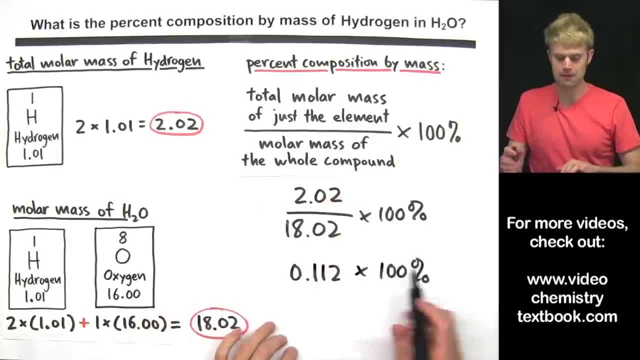 I'm rounding this to three significant figures because of this number up here And now. when I take this And multiply it by 100%, it will move the decimal two spots to the right. so I'll get 11.2.. And we'll also turn this into a percentage. 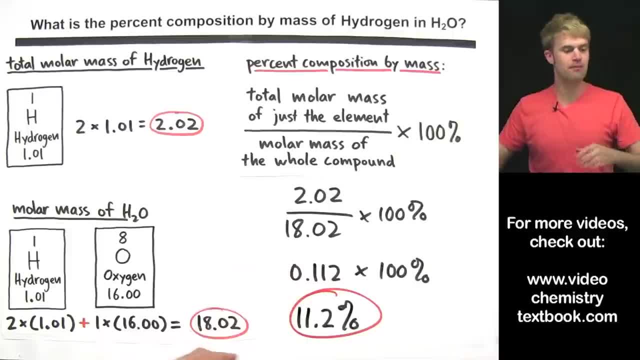 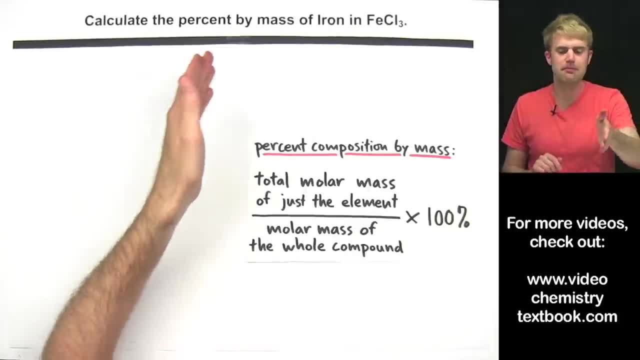 So 11.2% is the percent composition by mass of hydrogen in H2O. Let's do a couple more: Calculate the percent by mass of iron in FeCl3.. We're going to want to get a number for both of these, okay. 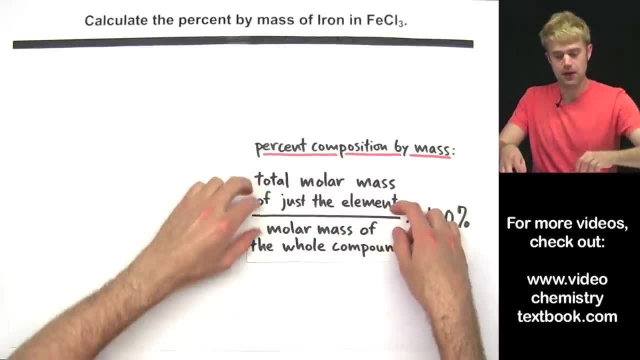 The total molar mass of just the iron, as well as the total molar mass of the hydrogen and the total molar mass of the hydrogen, And now we can use the formula to determine whether we have 1.7. whole battle for the ego. 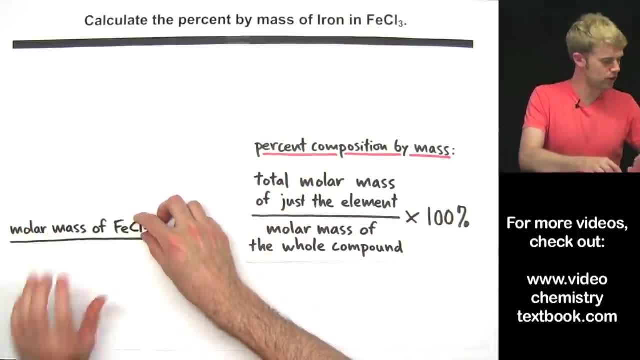 vtm. So for example, for theiffs we can say: there's a cost of this mercury, That's b in k格cM. Let's write it down. We've done that. oneizaD means we've made this very simple. Let's see if we have any problem with that. but let's enter in the value of the republican character. Is fdCl3 Greek schladza, three phdCl3 of go on, an array of going on. anpled is how us. 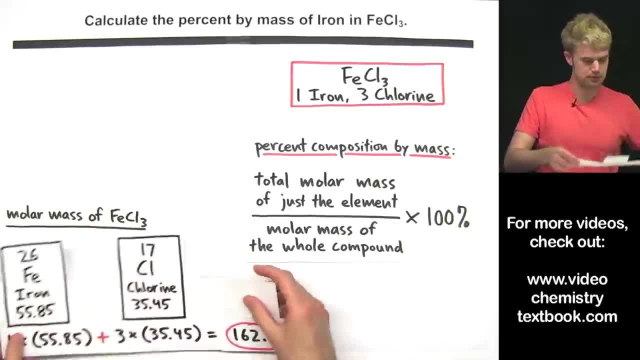 they look like bthe. сначала we have the molar mass of the whole compound, FeCl3.. Let's start out by determining the molar mass of FeCl3.. We look at the chemical formula. It tells us that we have one iron and three chlorines. 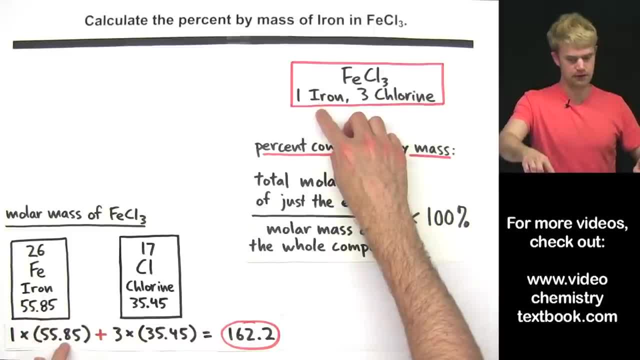 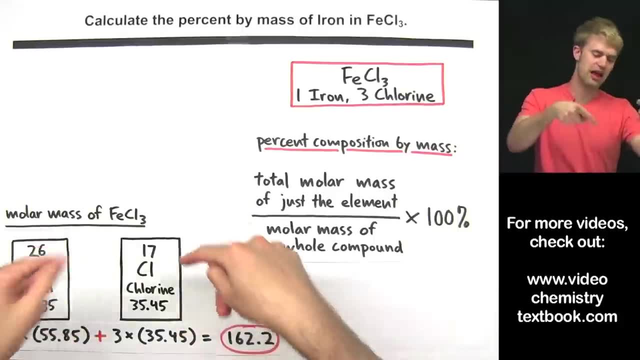 So we can take a look at the periodic table: one times the molar mass of iron, because we got one of them. three times the molar mass of chlorine, because we got three of those, and get this number for the total molar mass of the whole thing, fecl3. 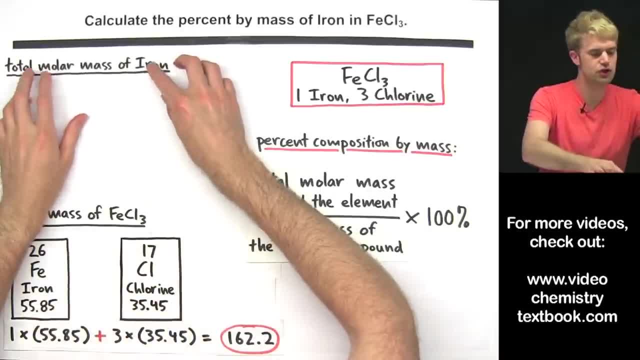 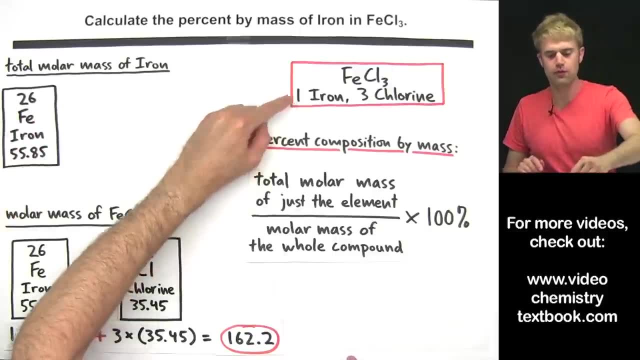 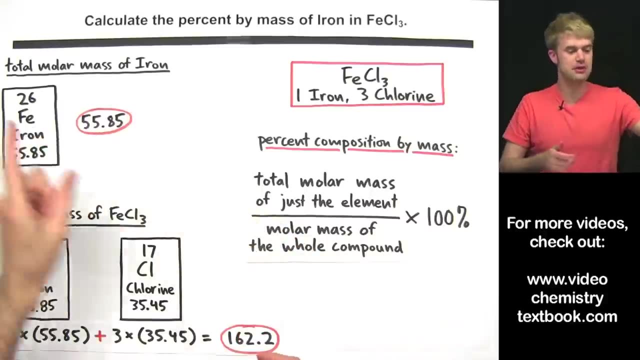 okay, now for the total molar mass of just the iron. we want to zoom in on iron. here's its molar mass. we look at the chemical formula and we only have one iron. okay, so the total molar mass of just the iron is going to be the same as just one iron: it's going to be 55.85. now we got the mass of. 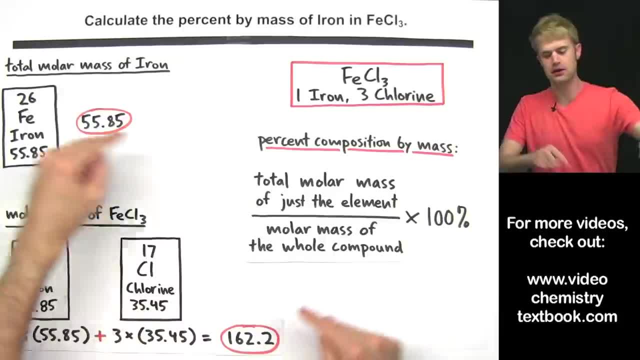 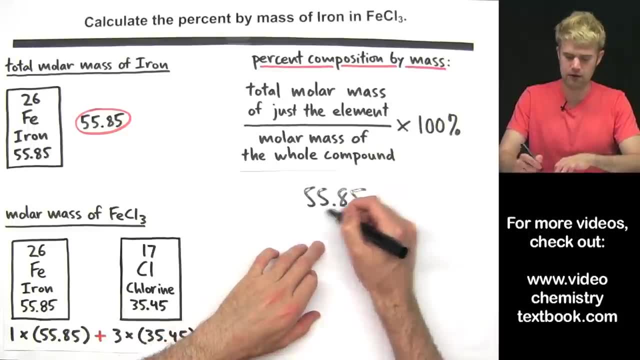 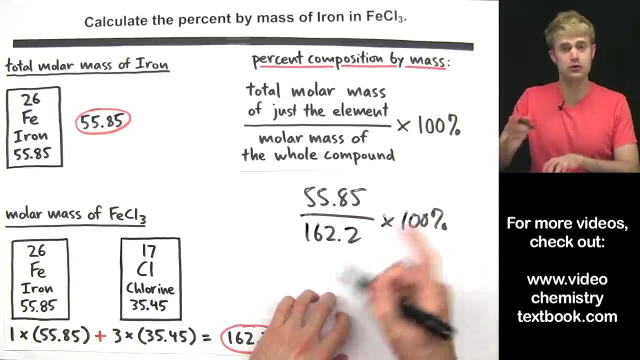 just the iron and we got the molar mass of everything together. let's put it in the equation: we'll take the mass of just the iron, 55.85, and divide it by the molar mass of the whole compound, 162.2 times 100. i'll do this in two steps. again, the first step gives me 0.344. 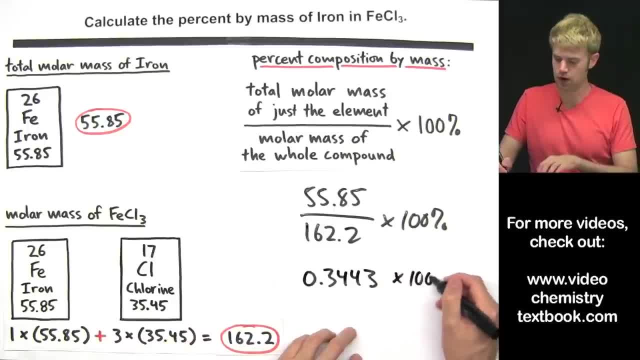 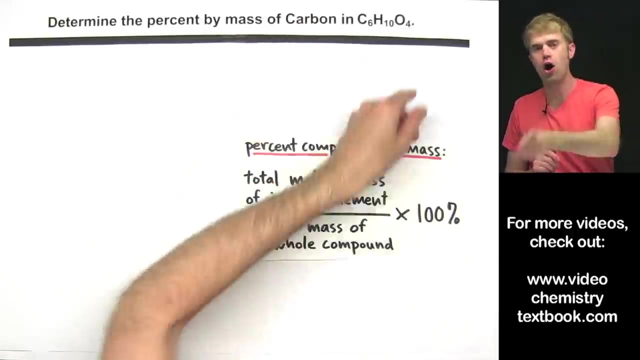 3 rounded to 4 significant figures times 100 percent and then multiplying this here we'll move the decimal place over two spots to the right, so i'll get 34.43 percent. the percent by mass of iron in fecl3 determine the percent by mass of carbon in c6, h10, o4- two things we want to keep. 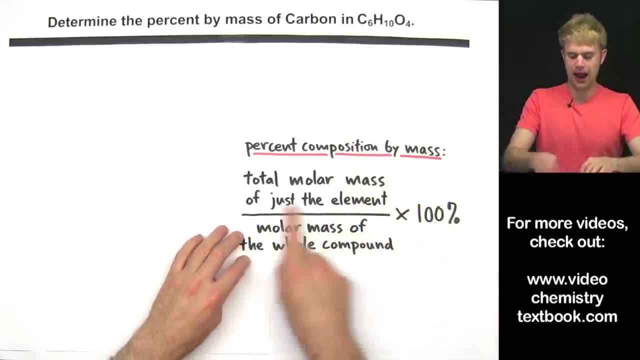 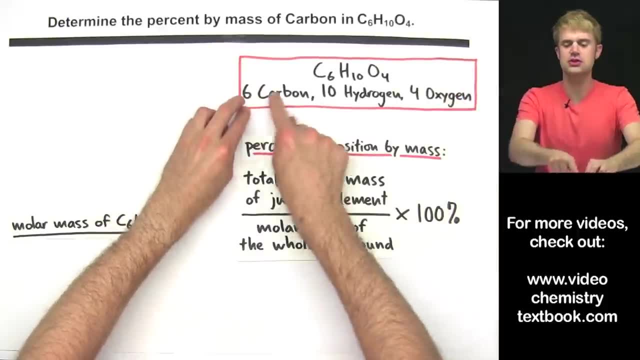 in mind the total molar mass of just the carbon and then the molar mass of the whole compound. we'll start with a molar mass, the whole compound, which contains six carbons, ten hydrogens and four oxygens. so we will add their molar masses. 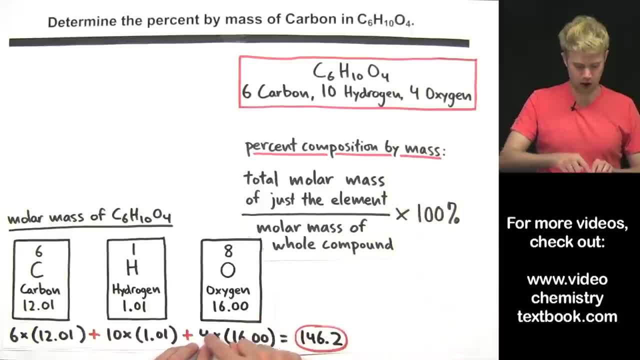 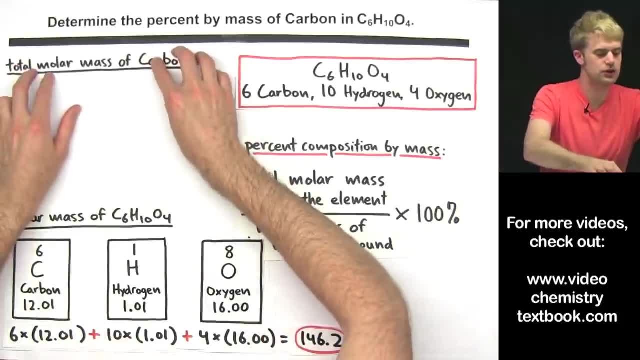 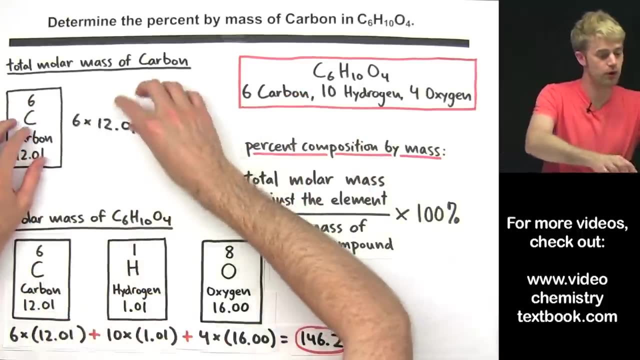 together six carbons, ten hydrogens and four oxygens and get 146.2 the molar mass of all of them added together. now, when we zoom in on just the carbon, we see that we've got six carbons here. so we'll do 6 times 12.01, which is how much one carbon weighs, and we get 72.06 the molar.